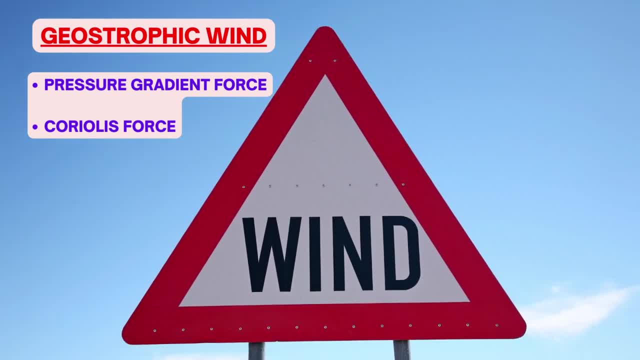 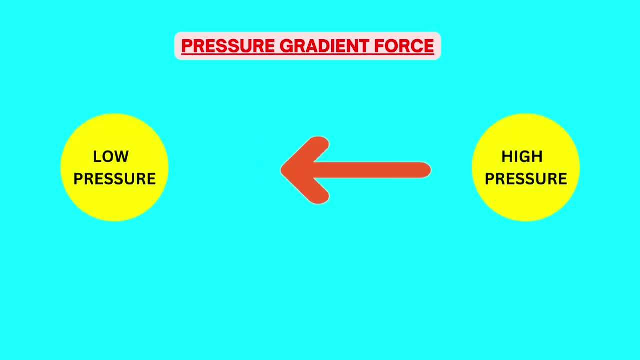 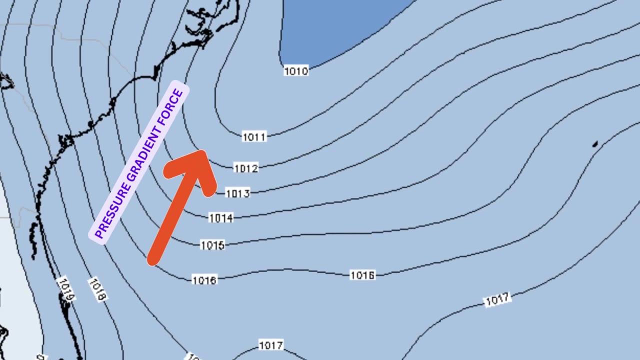 situation when only pressure gradient force and Coriolis force are present. Pressure gradient force is created due to pressure difference between two places or areas. So closer the spacing between two isobars, higher the pressure difference and higher the pressure gradient force and stronger will be the wind speed. Wind start blowing from high to low pressure. 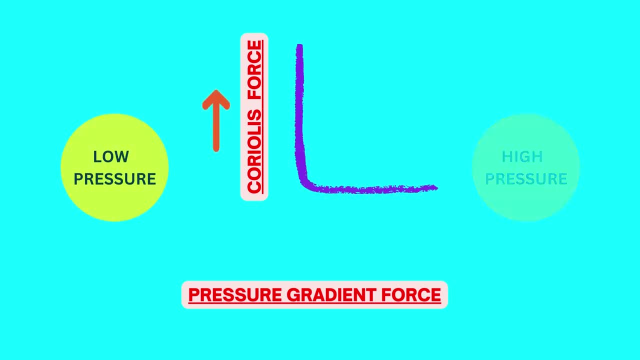 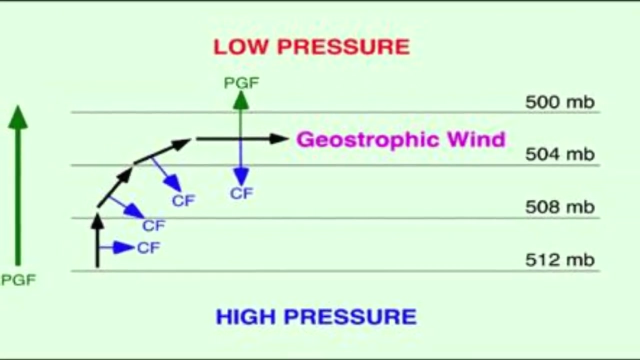 area. Within 24 hours, under the influence of Coriolis force, it starts curving to the right in northern hemisphere and to the left in the southern hemisphere and finally it gets parallel to isobars. Pressure gradient force and Coriolis force balances out each other. Wind direction. 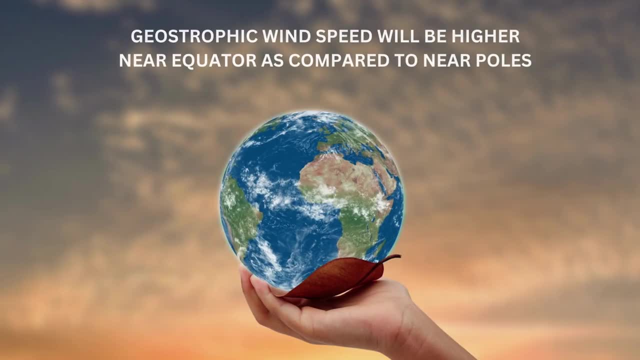 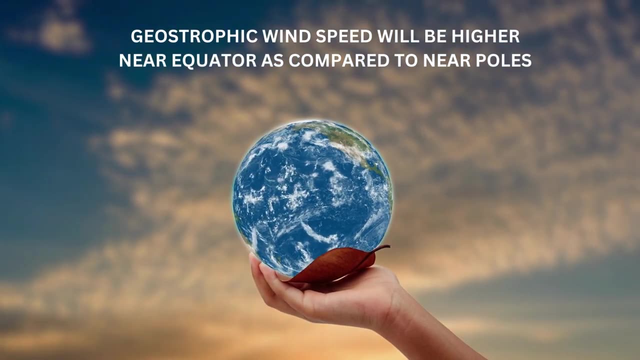 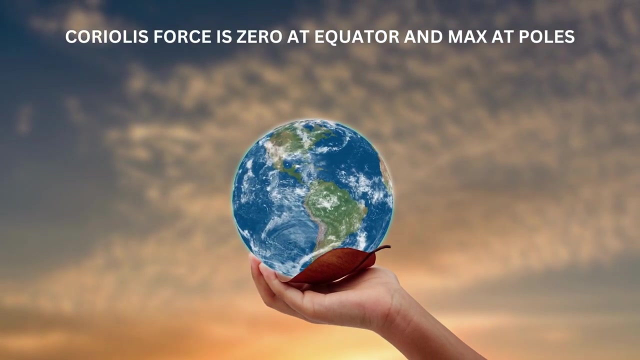 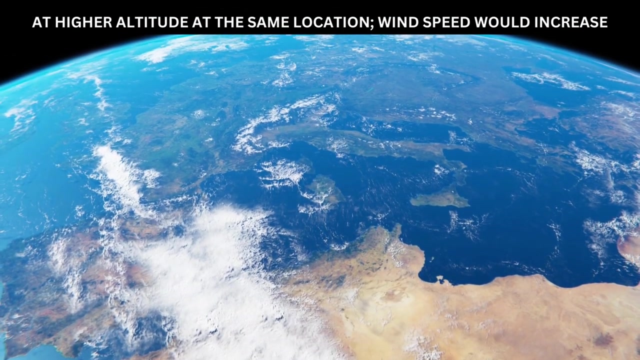 is straight and parallel along parallel isobars, Geostrophic wind speed will be higher near equator as compared to near poles for the same pressure difference. since Coriolis force is weak near equator For Geostrophic winds as you go to higher altitude at the same location, wind speed 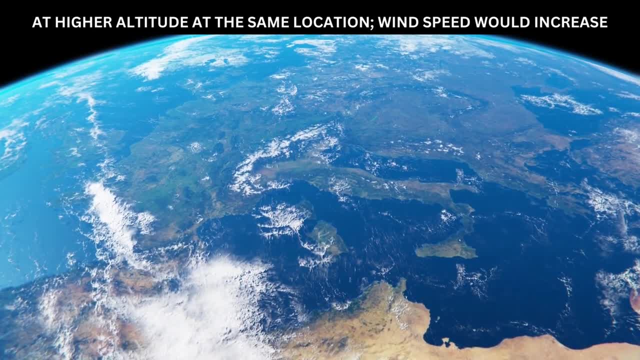 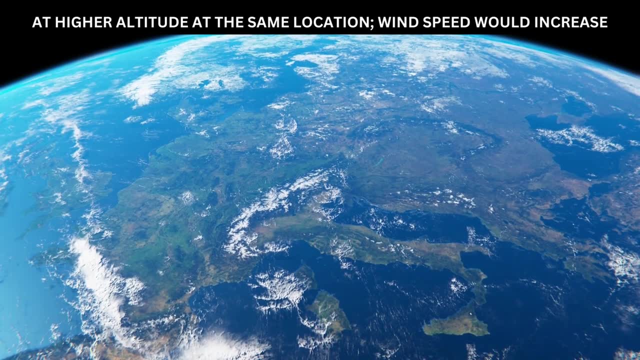 will increase. This is due to the fact that atmospheric density reduces as you go higher, so less resistance to the motion of the wind and hence higher will be the speed of winds. Geostrophic Wind. Wind is considered to be geostrophic above friction layer. 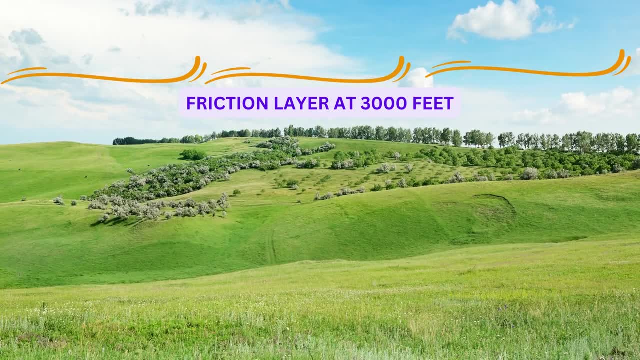 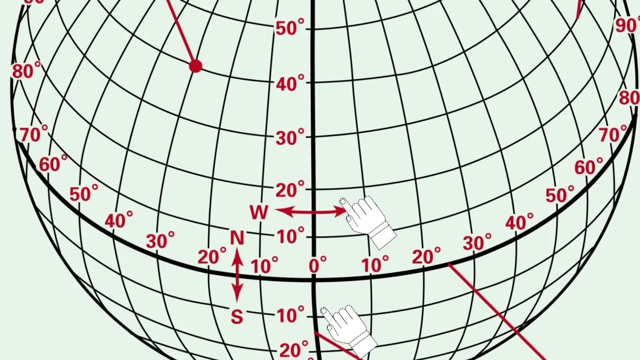 It starts from 2000 to 3000 feet and goes all the way up to tropopause. Since below friction layer, due to local conditions, terrain and obstructions, the mathematical modeling will not work out and will give incorrect results. Further wind is considered to be geostrophic only above 15 degree north and below 15 degree. 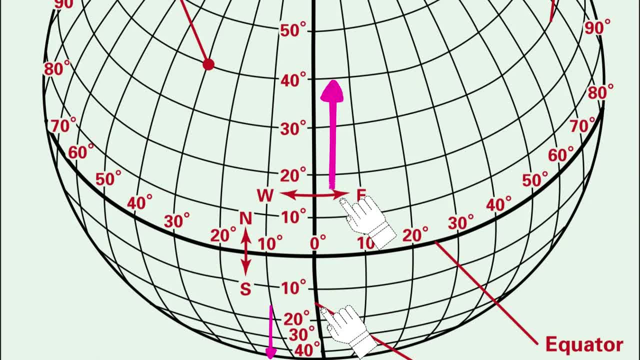 south latitude. Since below 15 degree latitude, the Coriolis force is considered to be negligible. Wind is considered to be geostrophic only above 15 degree north and below 15 degree south latitude. Since below 15 degree latitude, the Coriolis force is considered to be negligible. 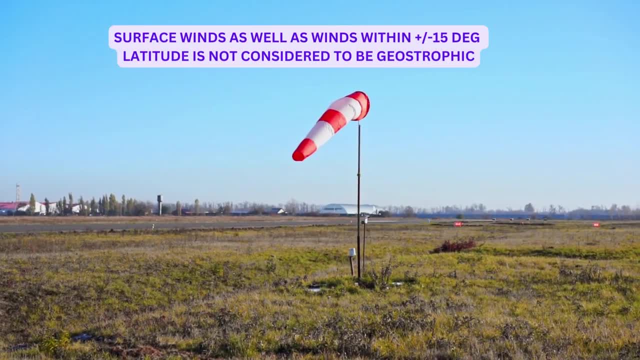 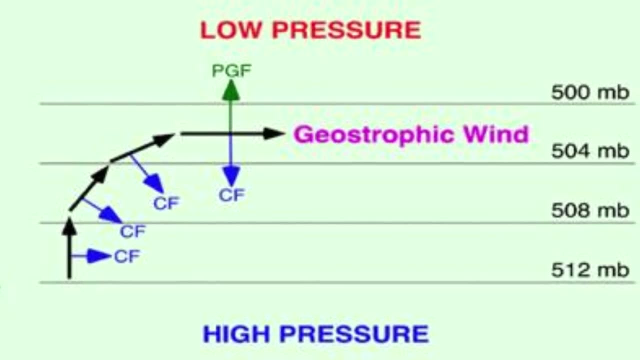 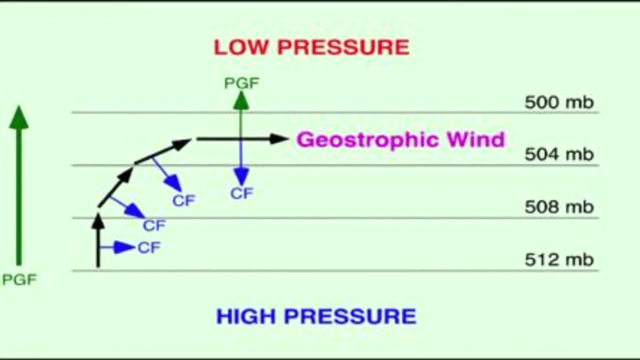 So the surface winds, as well as winds within ±15 degree latitude, is not considered to be geostrophic. Geostrophic wind will always blow along straight and parallel isobars under the balanced forces of pressure, gradient force and Coriolis force. 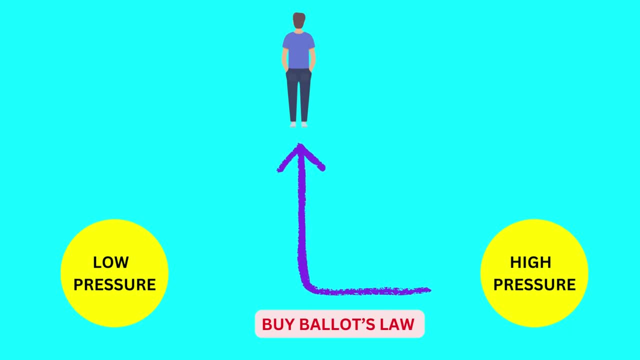 Wind direction can be found using by Belot's law, which states that if an observer is standing in northern hemisphere with his back towards the wind, the low pressure area will be on his left and reciprocal will be the result. in the southern hemisphere, questions invariably come during. 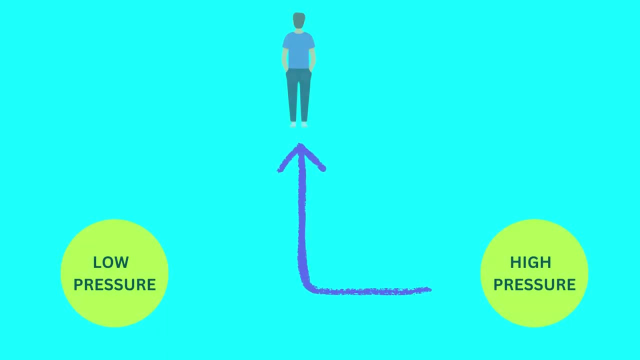 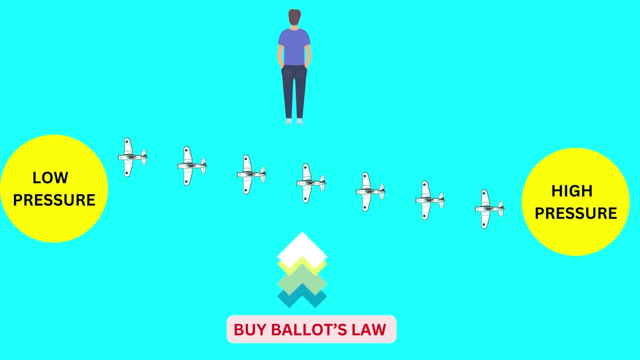 examination on interpretation of bybelot's law and sometimes the question is twisted in terms of port or starboard drift of the aeroplane, which can be walked out using wind direction. so in northern hemisphere if aeroplane is experiencing a startboard starboard drift, he is flying towards. 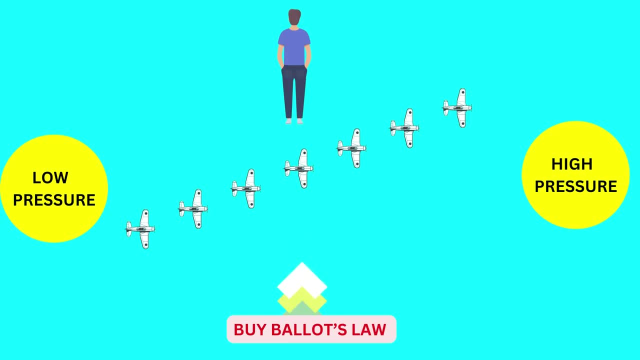 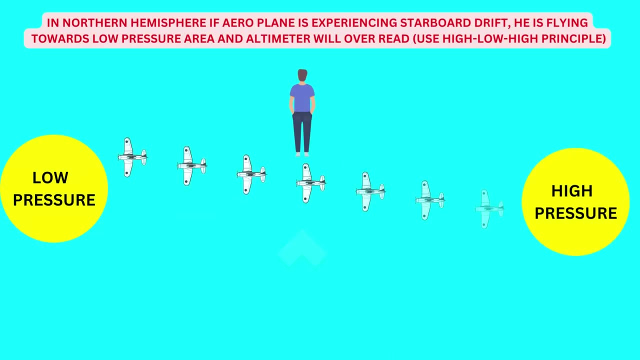 low pressure area and if he experiences a port drift, then he is flying from low to high pressure area. we can add one more twist to this question on altimeter reading. so in northern hemisphere if aeroplane is experiencing starboard drift, he is flying towards low pressure area and altimeter. 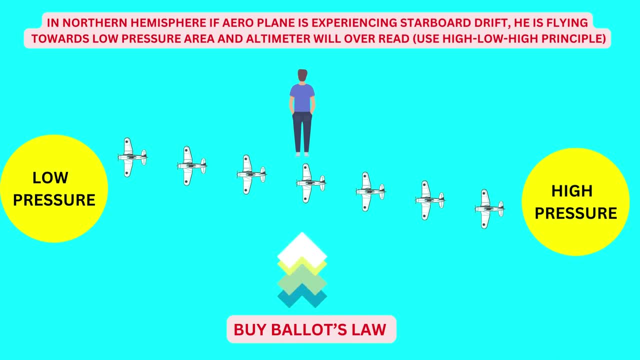 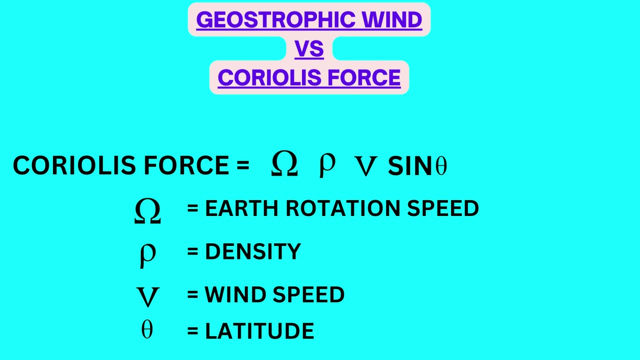 will over read and you can make out this by using high, low, high principle, so a lot of variable can be injected for questions on bybelot's law. geostrophic wind versus coriolis force. the formula for coriolis force is as shown on the screen. it is important to remember this formula, since this can help you in answering. 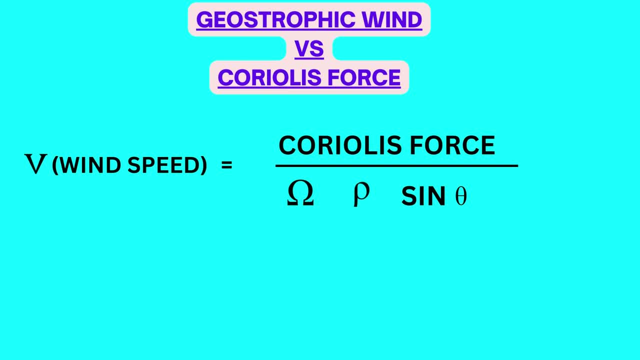 questions related to effect of latitude and density on wind speed. from this formula it is evident that for a given value of coriolis force, wind speed will increase if the latitude is lesser, that is, near the equator, and the if the density is lesser than the air cold zar. 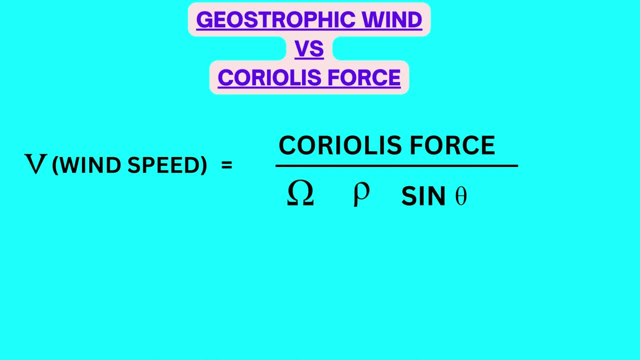 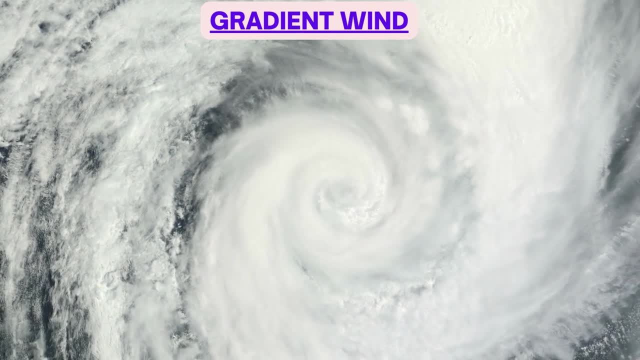 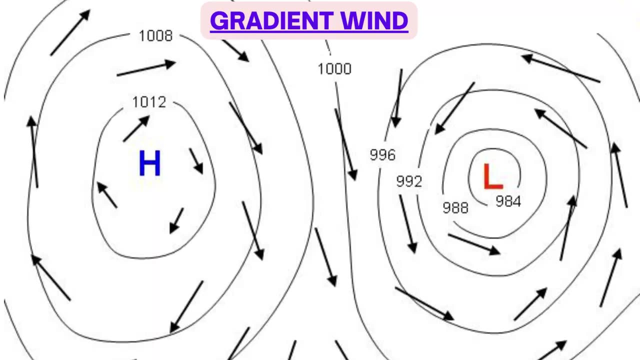 that is at higher altitude. now, moving on to the gradient wind. the gradient wind is the mathematical modeling of winds blowing in and around curved isobars, like in cyclone or anticyclone, and where there is a curved or circular motion involved, centrifugal force comes into play. centrifugal 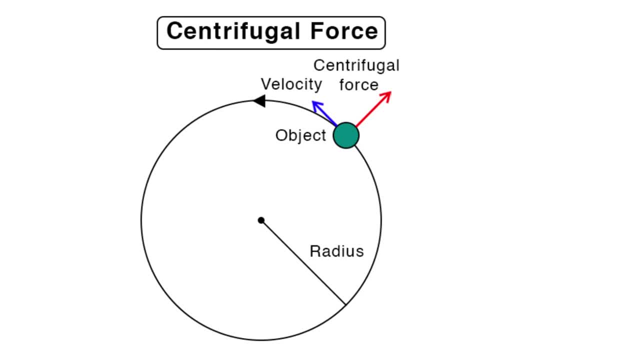 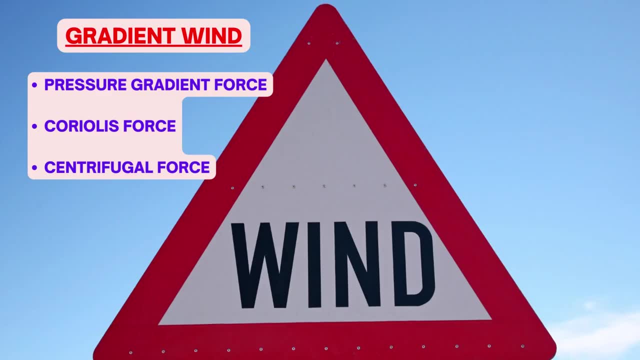 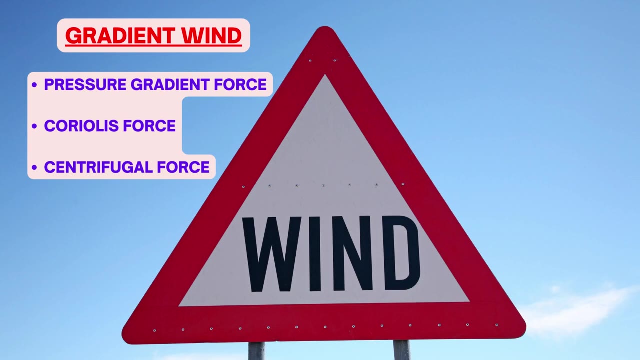 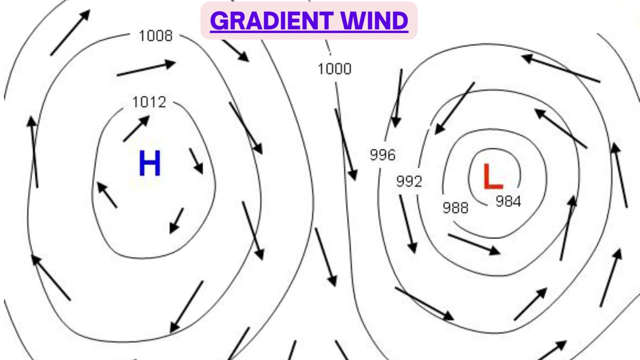 force is experienced by all objects moving in circular path, which tends to push the object radially outwards from the center of the circle. so gradient wind blows under the influence of three forces: pressure, gradient force, coriolis force and centrifugal force. wind blows parallel to isobars but follows a curved path, not a straight path. in gradient wind there are three forces. 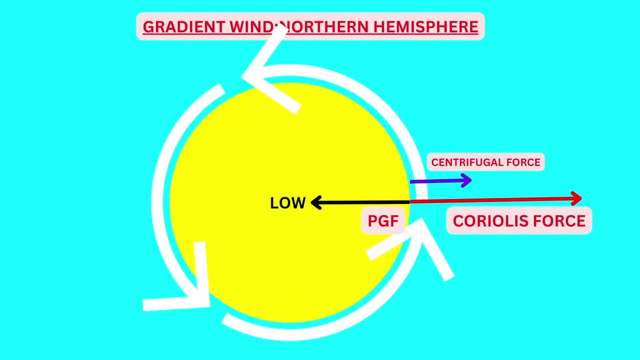 pressure, gradient force and coriolis force will always oppose each other, but centrifugal force will assist or add to the coriolis force in a cyclone, low or a depression, and oppose the coriolis force in an anticyclone or high. so this additional centrifugal force will tend to slow down the speed of winds in a cyclone. 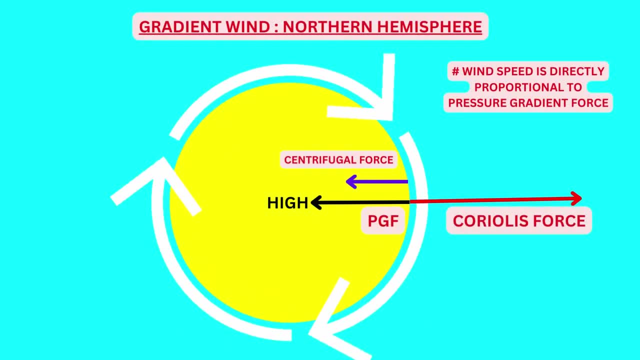 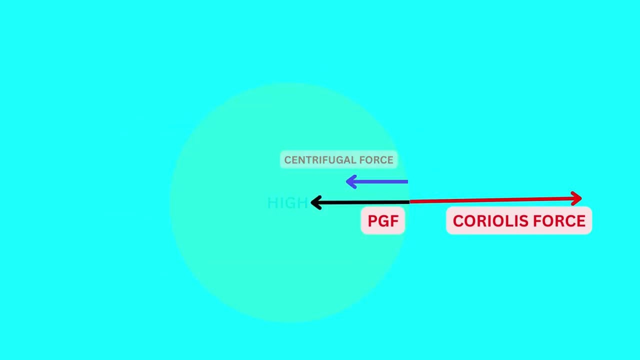 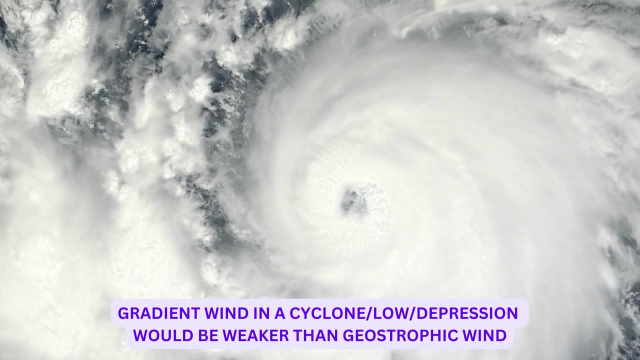 low or depression and accelerate the wind speed in an anticyclone or high for the same given pressure. gradient force question can be based on this effect of centrifugal force on wind speed. so gradient wind in a cyclone, low or a depression would be weaker than geostrophic wind and gradient. 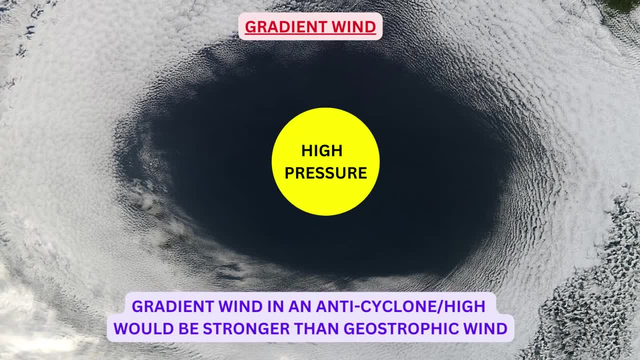 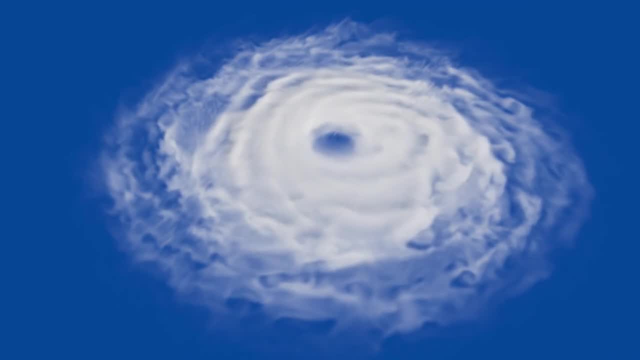 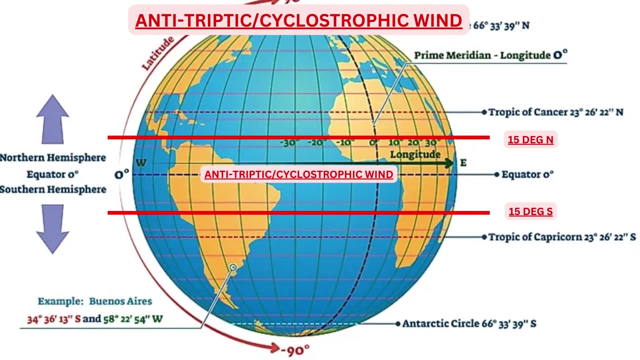 wind in an anticyclone or high would be stronger than a geostrophic wind. this does not mean that the both type of wind is blowing at the same time. it is just that which wind modeling will give you what kind of prediction for wind speed: antitryptic wind or cyclostrophic wind, geostrophic or gradient? 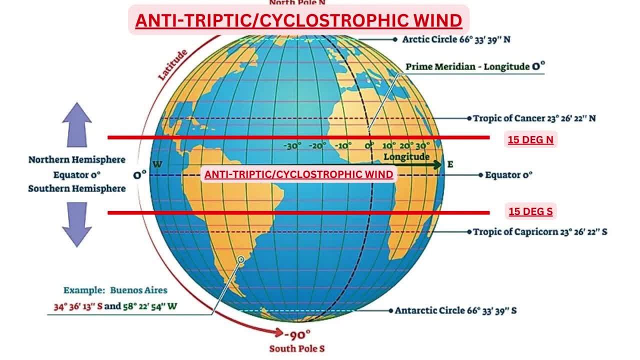 wind. for both of them to be modeled, presence of coriolis force is mandatory. so what about the winds in geographical areas within plus minus 15 degree latitude from the equator, where coriolis force is close to zero? so, winds within plus minus 15 degree latitude from the equator where coriolis force is. 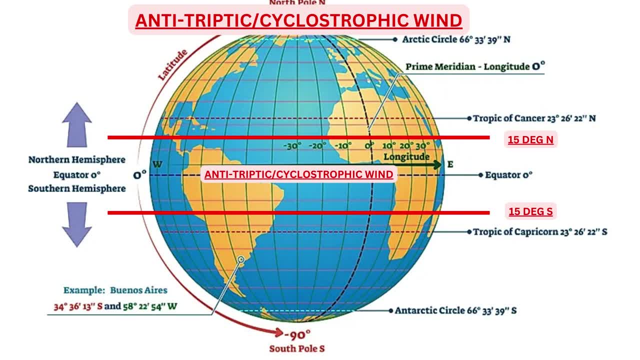 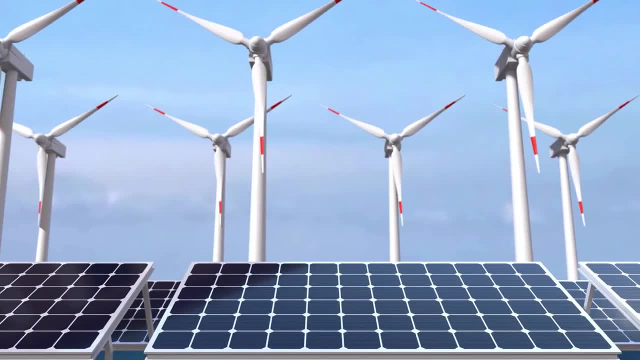 negligible, is called anti-triptych wind or cyclostrophic wind. so hope this video has helped you in understanding the topic of geostrophic wind in a cyclone, low or a depression or a depression with absolute clarity. with this we have arrived at our destination. subscribe the channel for more. 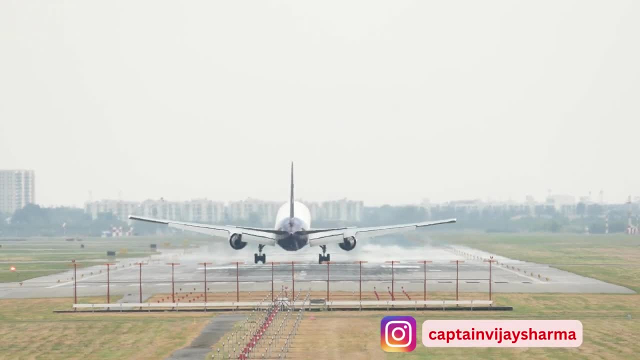 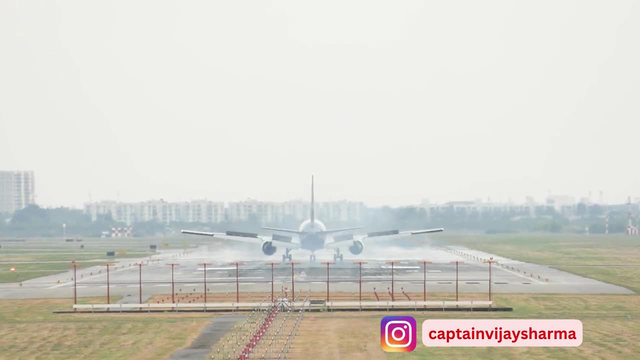 such informative videos on aviation, follow me on instagram link as shown on the screen. do not forget to comment below: did you like the video or if you want me to cover a specific topic? hope to see you on board again for the next flight. till then, happy landings. you.